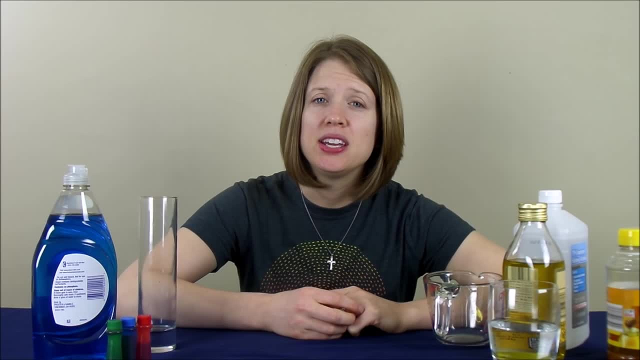 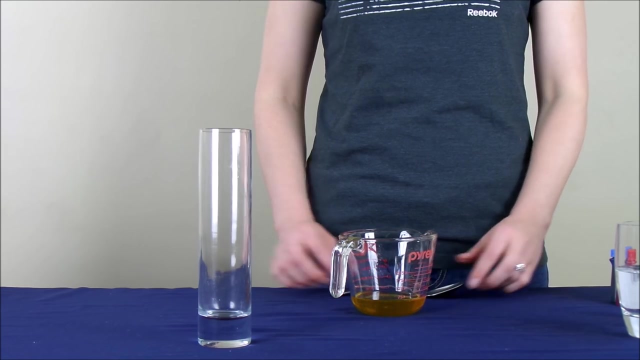 Hey everybody. it is Danielle from Cool Science Experiments headquarters. Today I'm going to show you a science experiment called Rainbow in a Jar. Are you ready? Let's get started. So the rainbow we are going to make is going to have five colors. It's going to go red, yellow, green, blue. 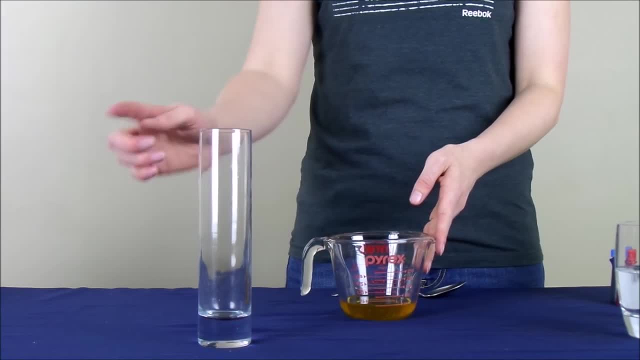 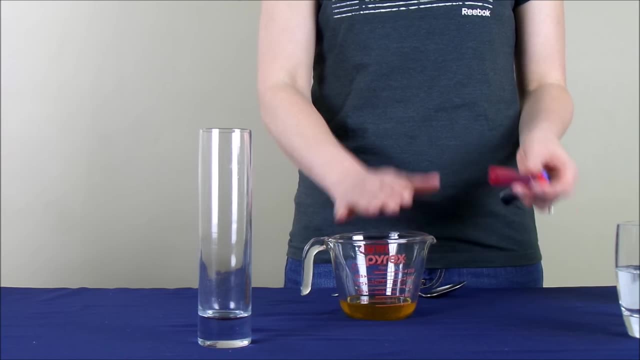 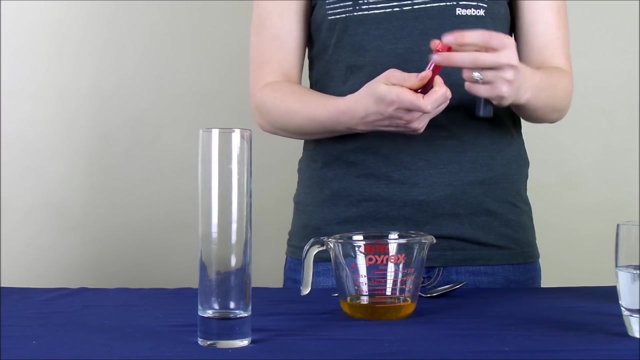 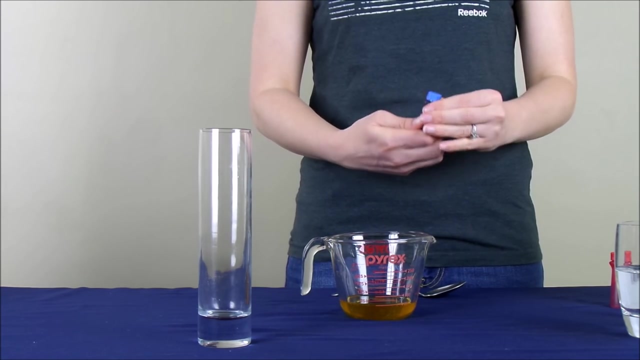 and purple. So we will start by pouring our purple color into the jar And what you need to do is get about a quarter cup of honey and add to it one drop of red food coloring and one drop of blue food coloring. Then you're going to mix it up and it's going to turn the honey. 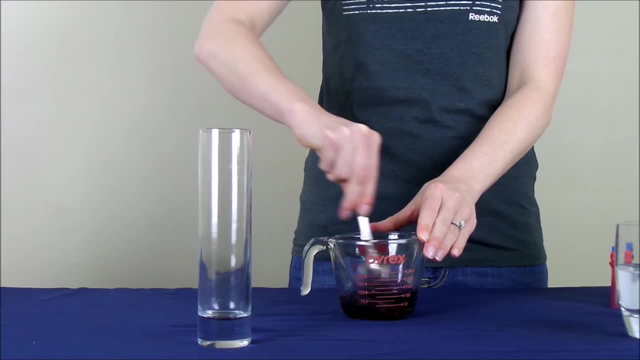 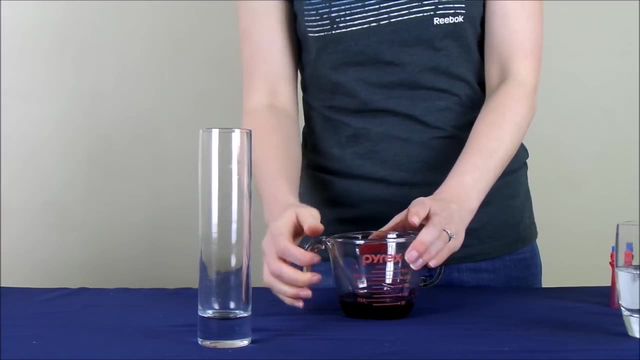 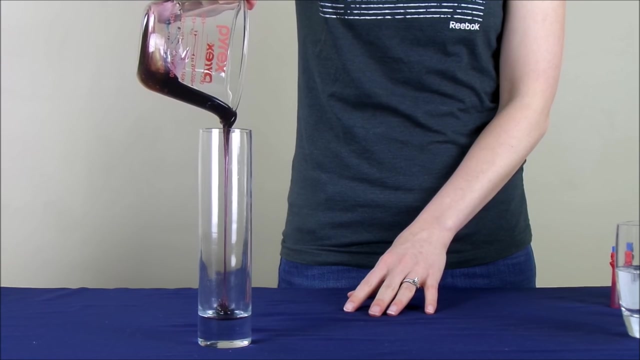 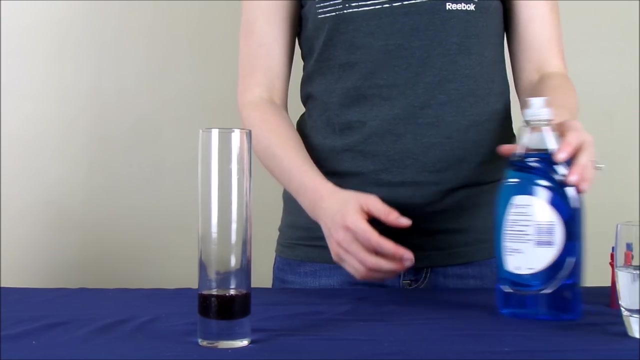 purple. So after you have your purple honey, you are going to pour it into your jar. So now that we have our purple in our jar, we're going to add a layer of blue and to do that, we're going to take some blue dish soap and we're going to 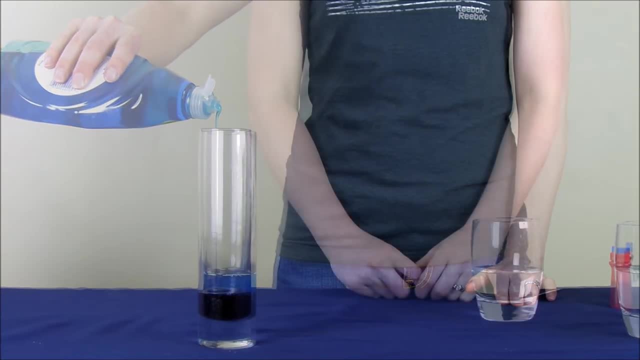 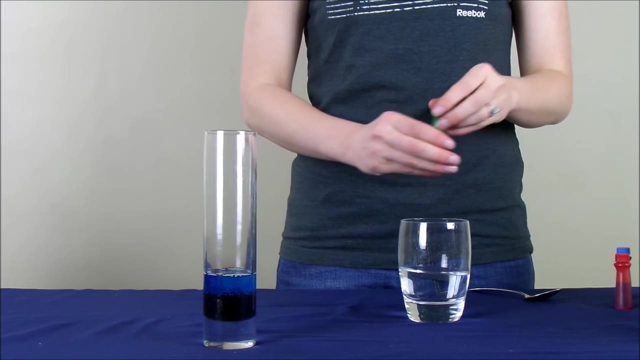 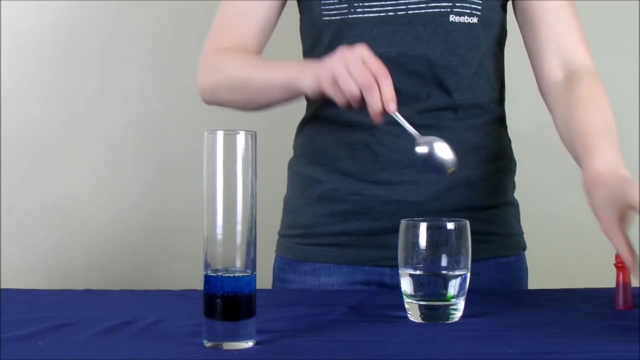 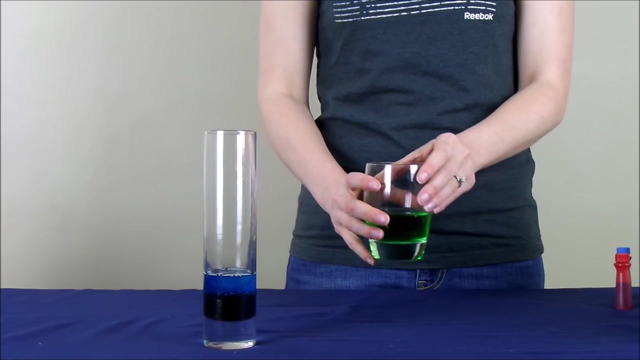 add it to our jar. Now we're going to move on to our third layer, which is green. To make the green layer, you take some water and you add a couple drops of green food coloring to it. You stir it up. You're going to want to be very careful. 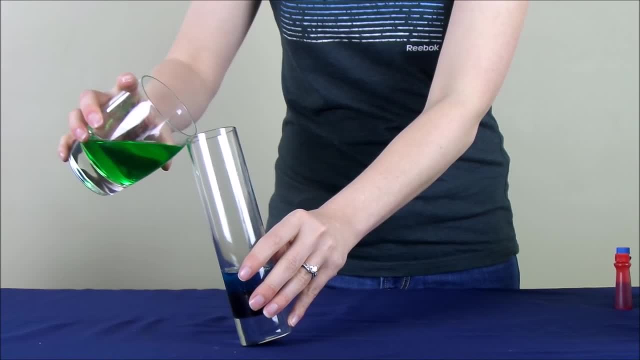 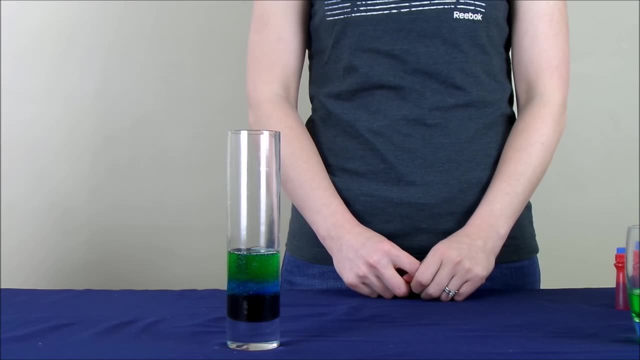 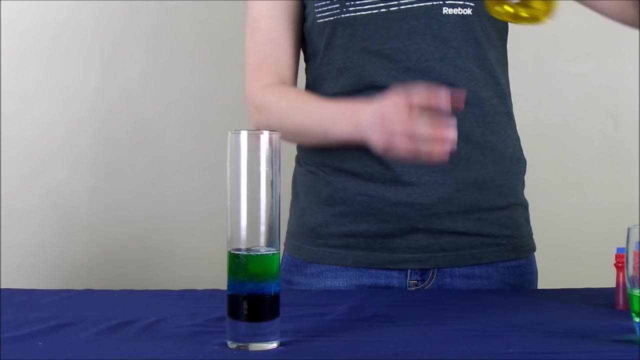 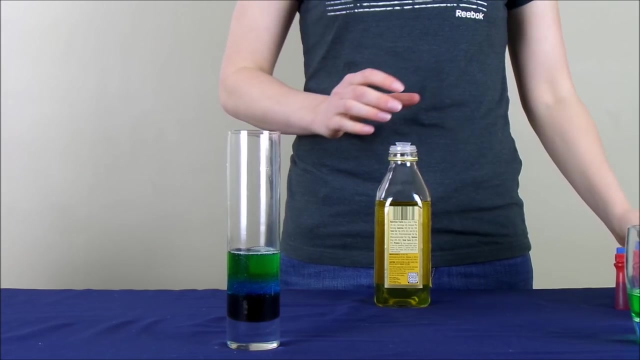 as you pour the water into the glass, I'm going to turn it on its side and just slowly pour it in. So, now that our third layer is complete, the next layer we are going to do is our yellow layer, and for that we are going to need some olive oil, And again, I'm